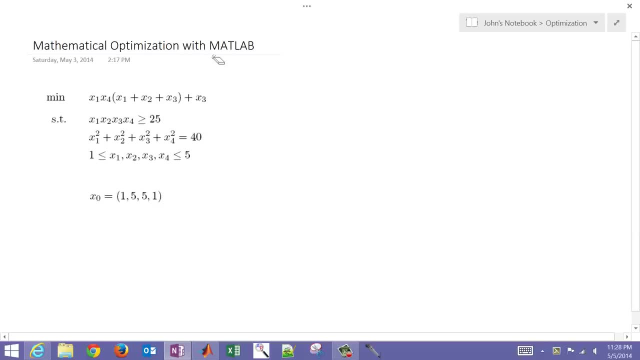 This is a brief tutorial on solving mathematical optimization problems with MATLAB. We're going to use an example problem, in this case with an objective function, a nonlinear objective function with four different variables. We have x1 through x4. And then we're also subject to so at the optimal solution. 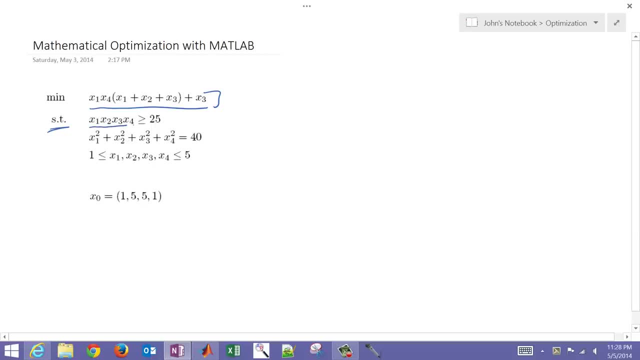 these constraints must be satisfied. We have that the product of all four of our variables has to be greater than or equal to 25. And then also the sum of the squares of those four variables has to also equal 40. The other thing that we have is these individual variables. 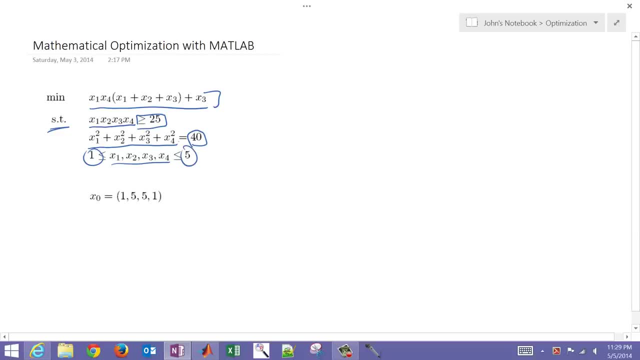 are constrained to have a lower bound of 1 and an upper bound of 5.. And then we're also saying that the initial guess for all four of our variables are 1,, 5,, 5, and 1.. And so that's going to be where we start our optimizer. 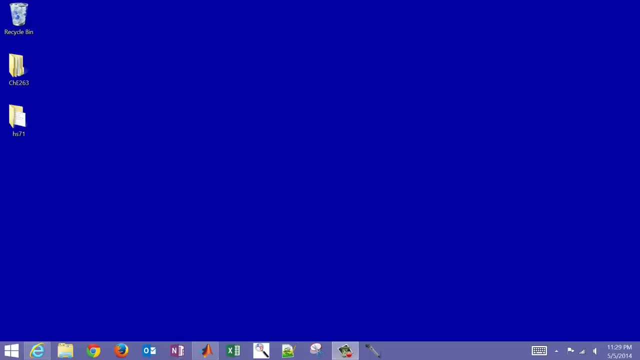 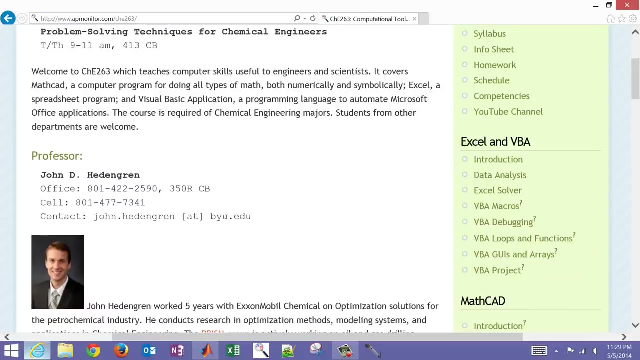 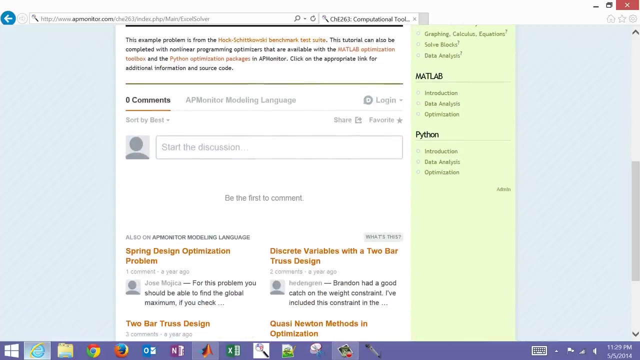 with our initial guess. So what I want to do now is come to the course website- This is Computational Tools for Engineers- And then we already covered this in Excel- the same problem on how to solve it in Excel- And then what we're going to do now is come down to the MATLAB section. 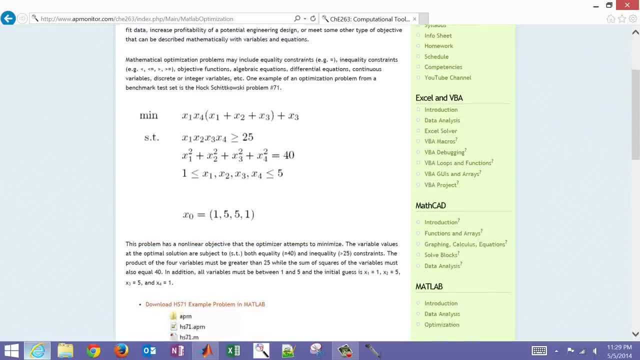 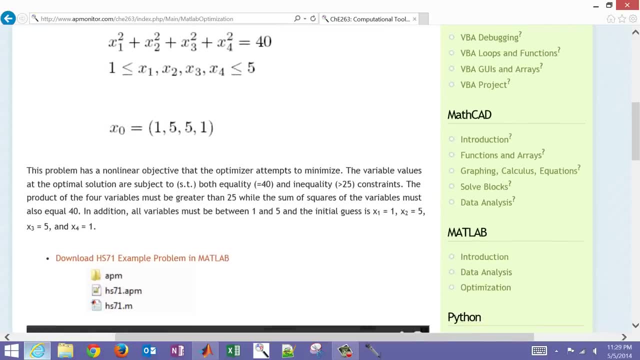 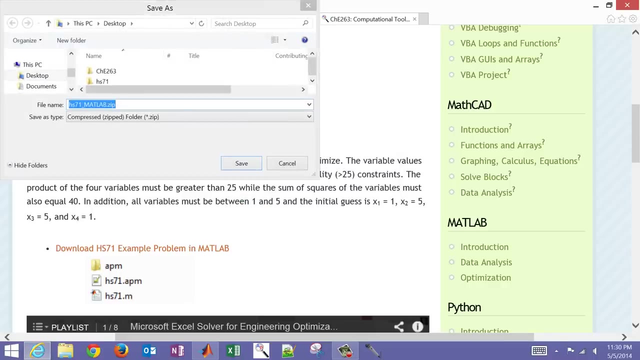 Now you can also visit the Python section as well. the same optimization problem. What we want to do is now just download this example problem in MATLAB. Okay, so let's go ahead and save it. I'll just go ahead and save it to the desktop. 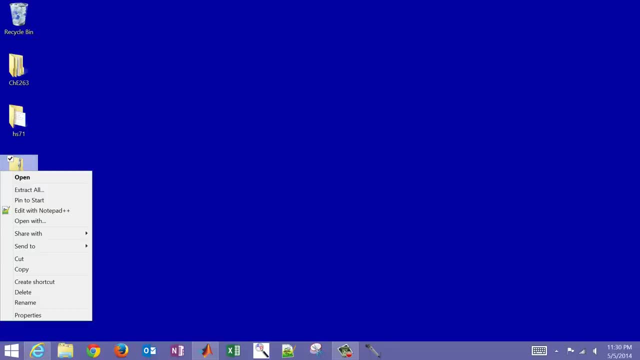 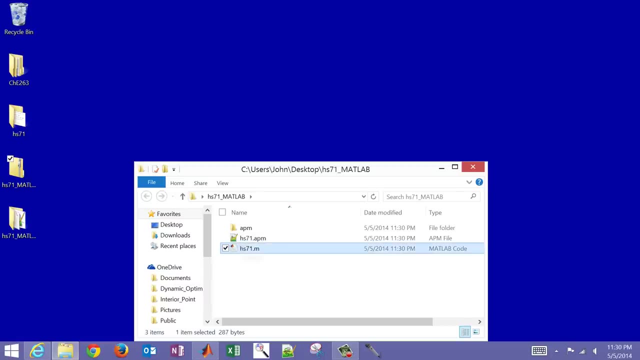 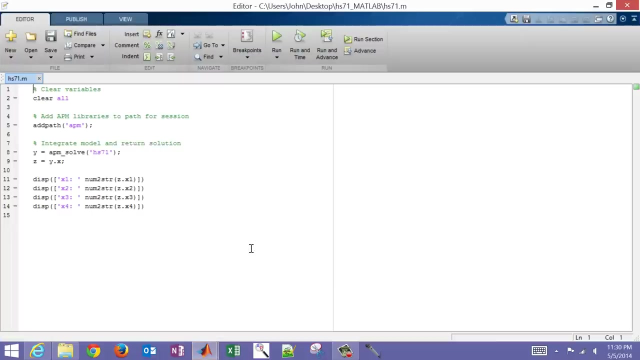 And then come over here and select it, extract it. It's important to be able to extract it. Sometimes MATLAB doesn't like it if you have it in the zip file And we have a script file here which runs our optimization problem. 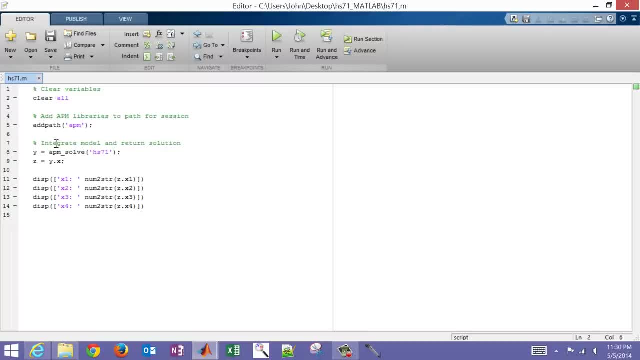 And so what it's doing is just clearing all the variables. It's adding the AP Monitor optimization toolbox And then it has the APM solve command with the name of our model HS71. And then it'll return the solution Y. 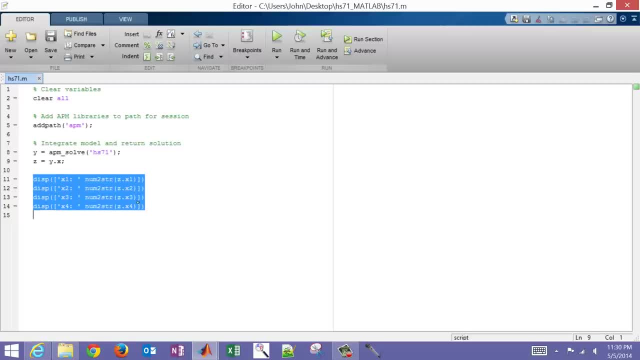 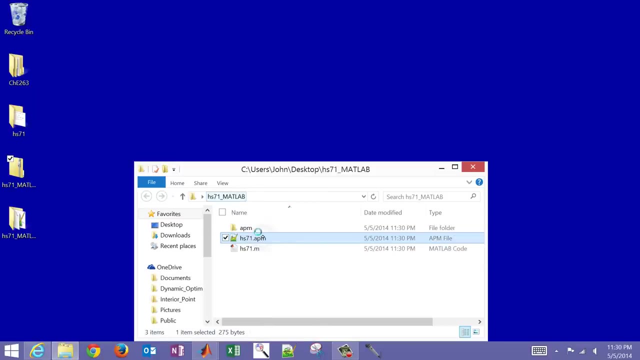 And then these last couple lines are just to extract the solution and be able to print out the solution to the screen. Okay, so let's take a look at this model file, the HS71 model file, And we have in here as well. now, this is in. you know, this is just any notepad.